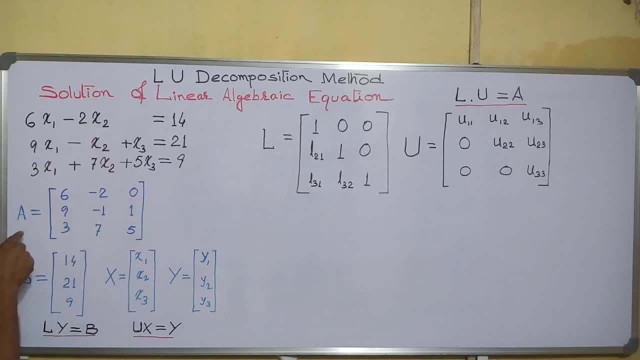 and this is the third equation. First write that a equals to the coefficients 6,, 9,, 3, minus 2, minus 1, 7,, 0,, 1, 5.. B is this equation: 14,, 21,, 9.. We are assuming x equals to x1,, x2, x3. 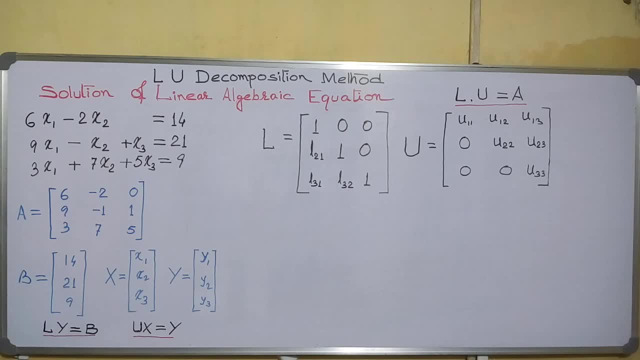 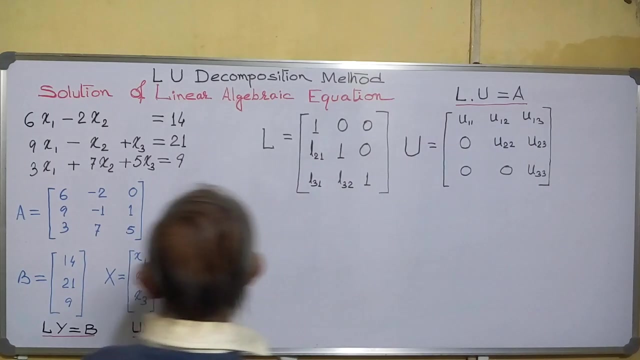 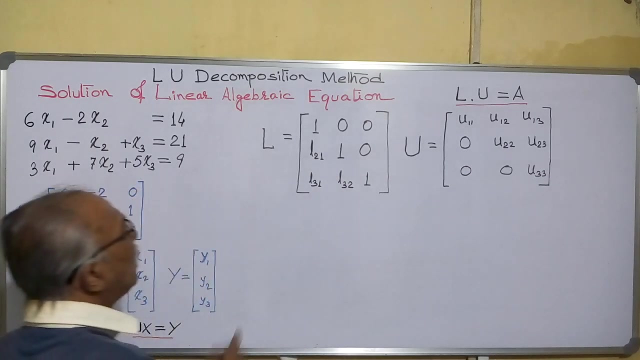 y equals to y1,, y2, y3.. The method we will apply here: ly equals to b and dx equals to y. First what we will do: l into u equals to h. This is our assumption. So we have to break this matrix into two matrix, such that l into u equals to h. Now let me. 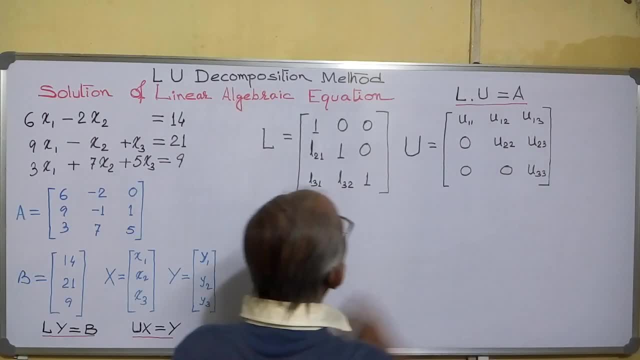 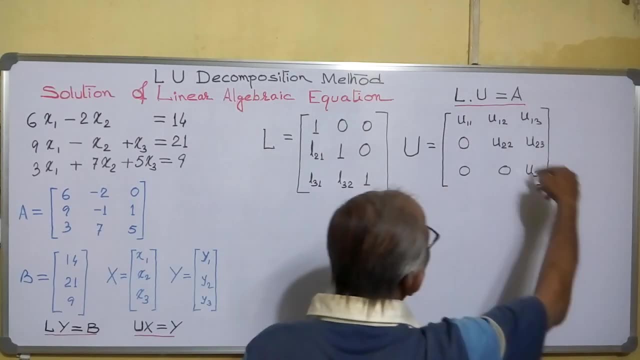 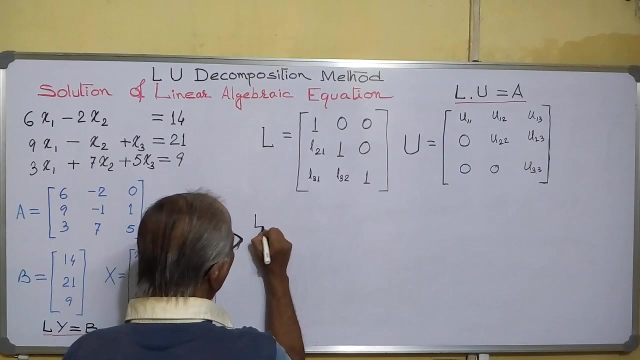 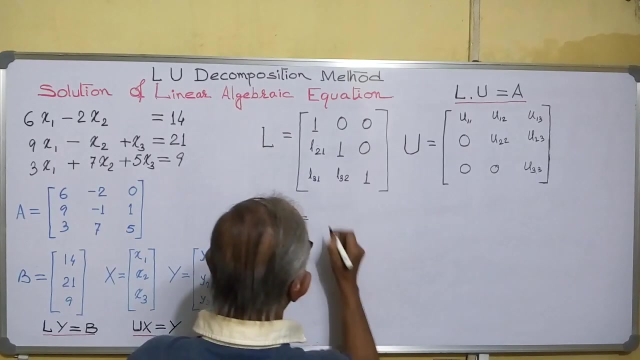 it is a lower triangular matrix and it is a upper triangular matrix. This 1, 1, 1. either you can take this here or here, Any one place you can take It is convenient to do. Now we find l into u, So l into u equals to first row, into first. 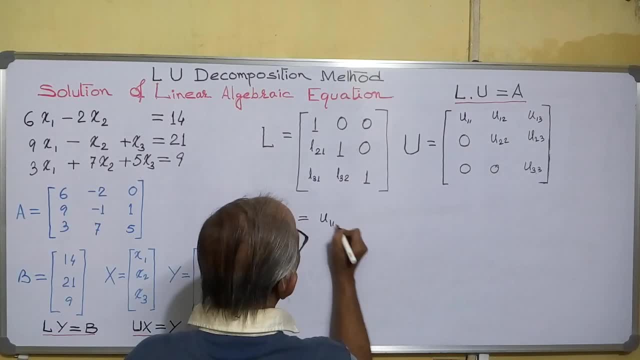 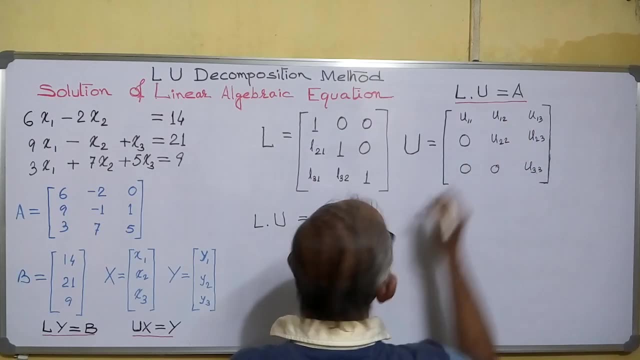 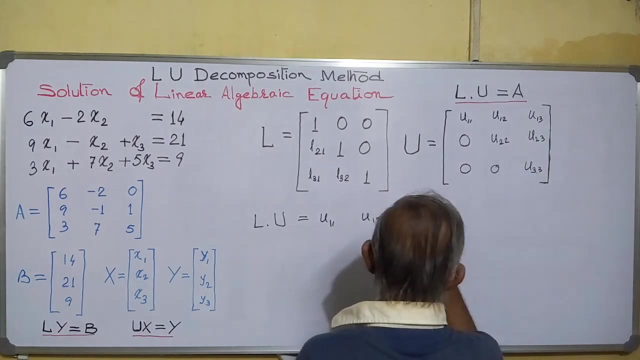 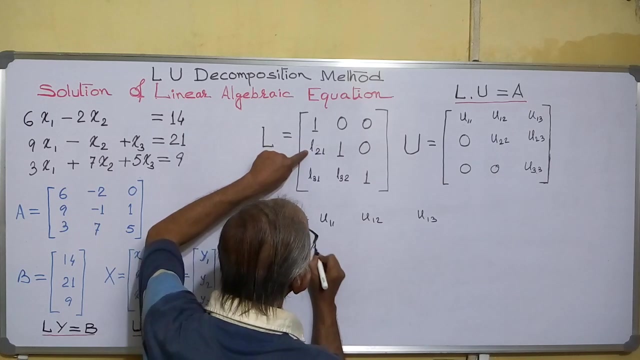 column u 1, 1, plus first row into second column, This will be u 1, 2.. Now first row into third column: u 1, 3.. Now second row into first column: u 2, 1,. u 1, 1.. 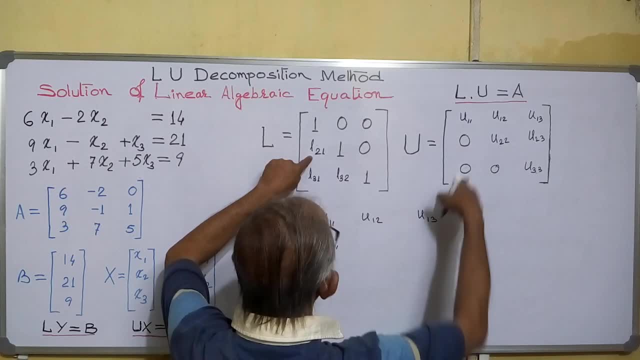 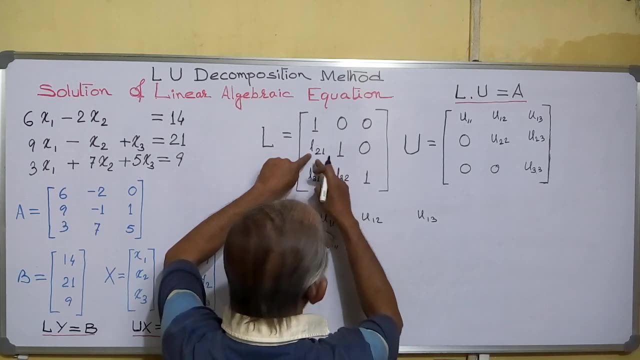 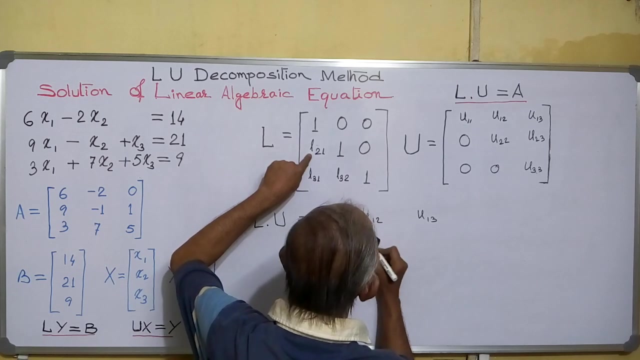 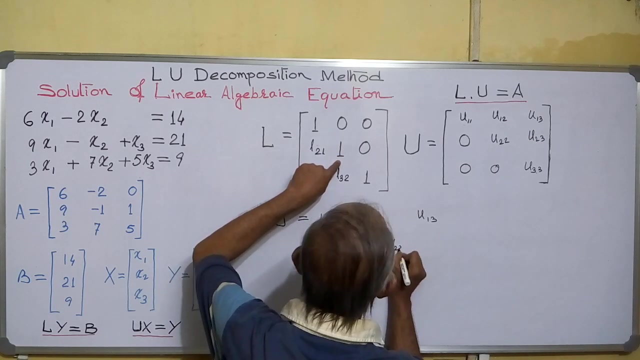 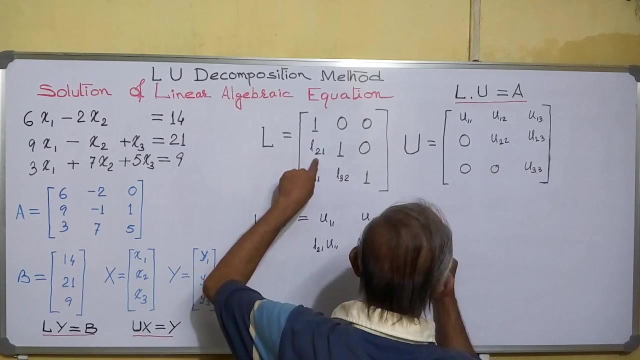 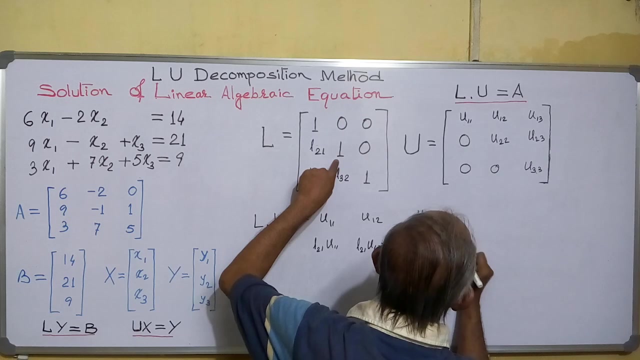 Plus all other things are coming together. Then second row into second column.03, 8, and 9.. L21, U12 plus U22.. You are knowing matrix multiplication. Now second row into third column: L21, U13 plus U23.. 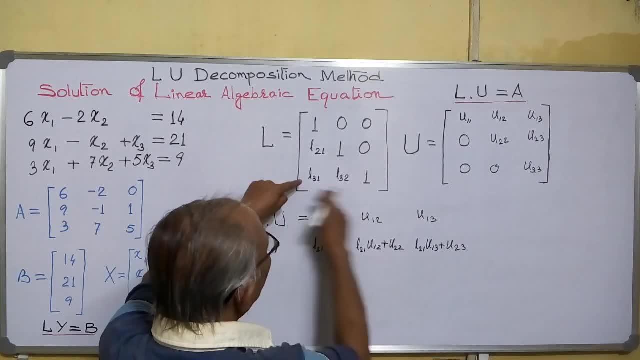 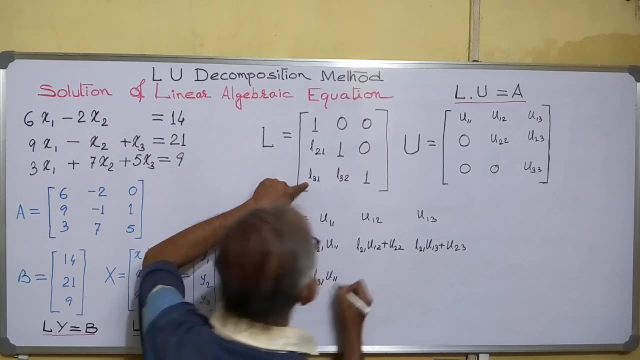 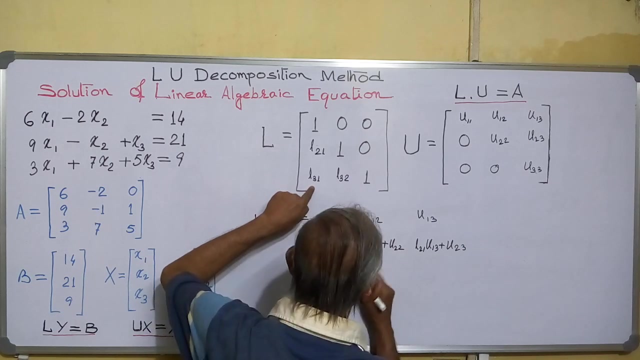 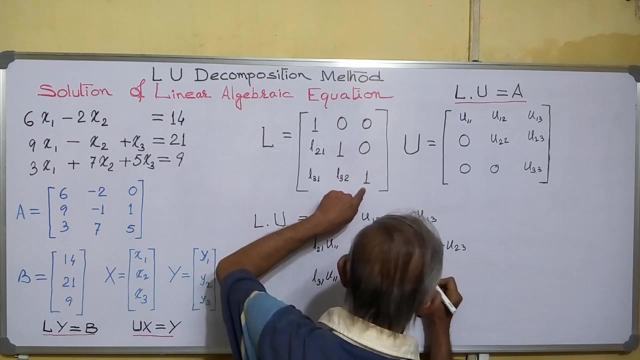 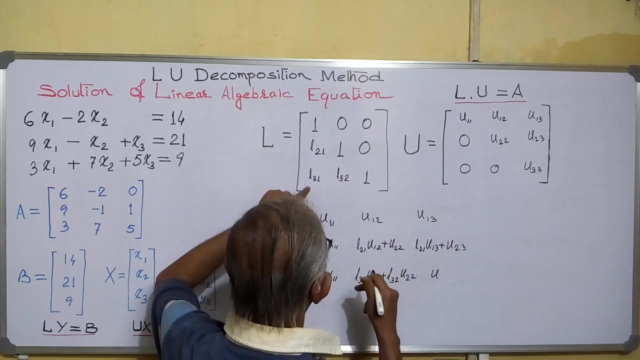 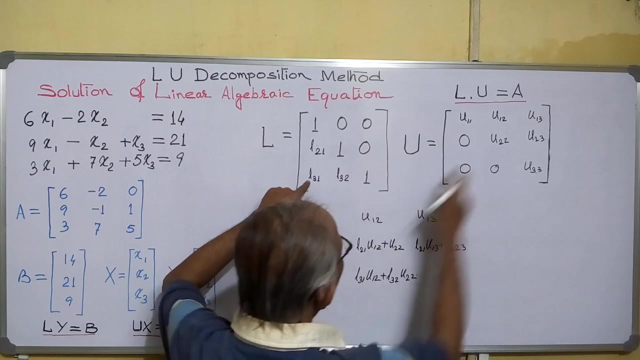 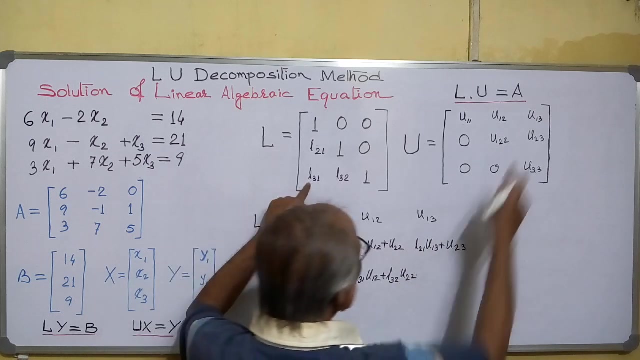 Now we come to third row into first column: L31- U11.. Third row into second column: L31- U12 plus L32- U22.. Plus U33.. Third row into N31- U12 plus N32- U22 plus 1 into 0 is 0.. Third row into third column. 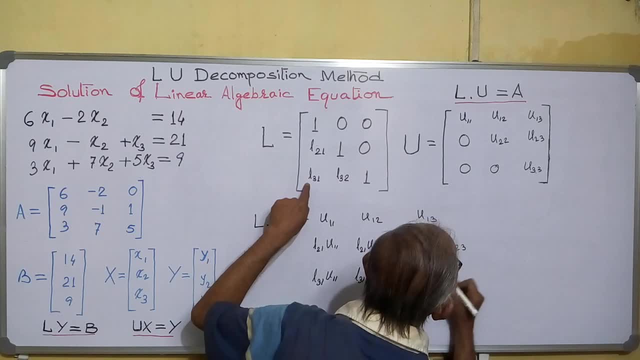 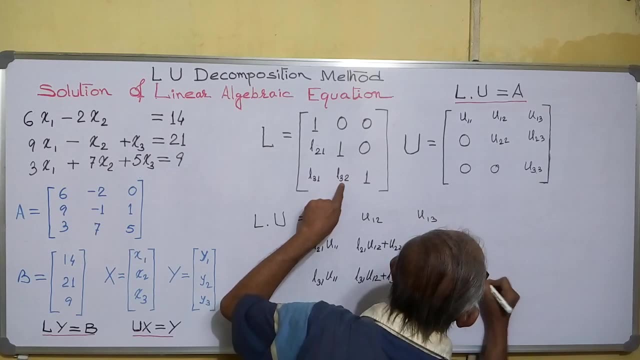 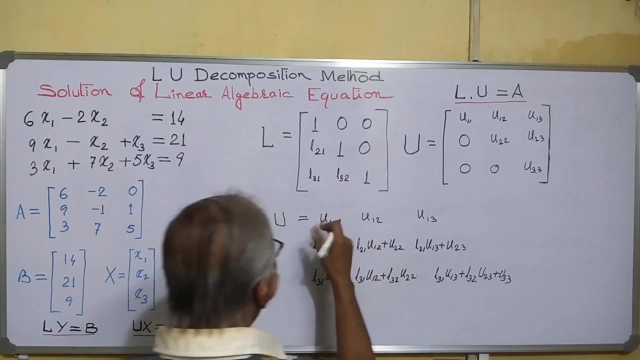 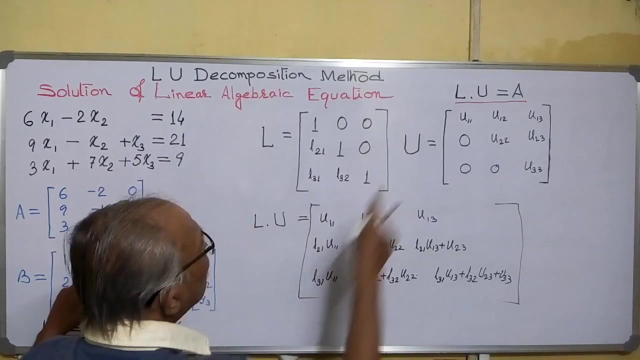 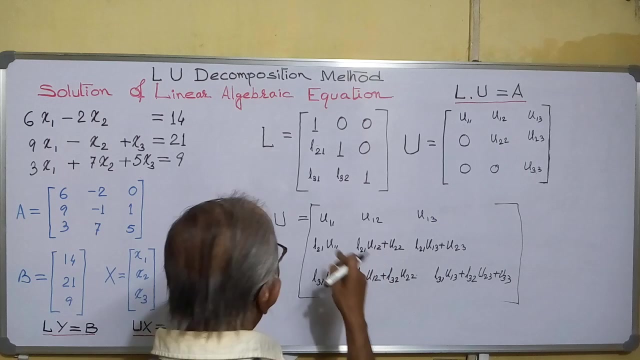 L31- U13.. Plus L32, U23 plus U33.. Now, by comparison, this is our LM matrix and this is equals to A. That is our assumption. L into U equals to A. We were searching that. what is L and what is U? 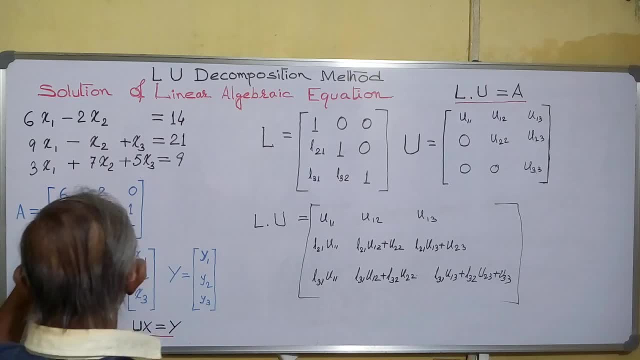 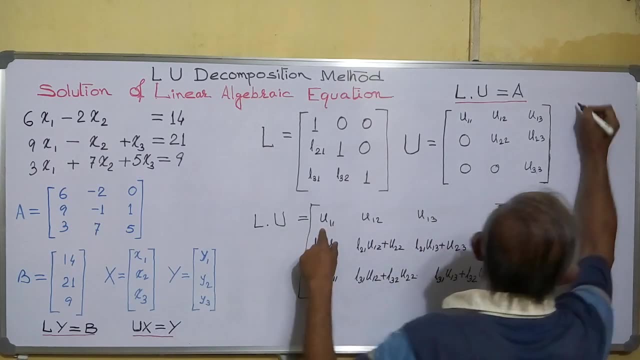 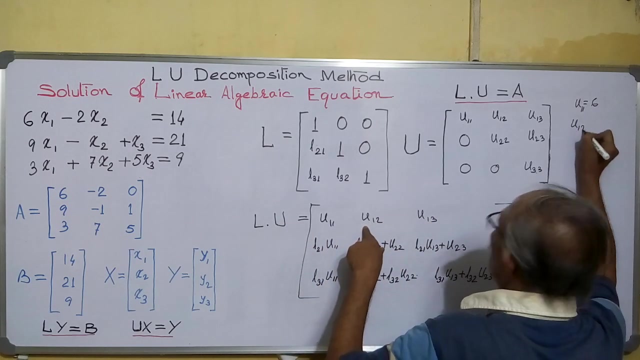 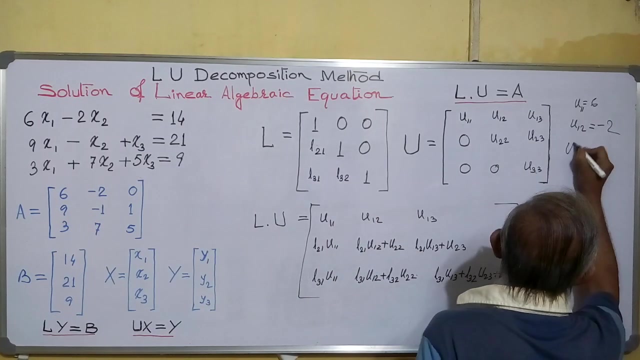 We got this And now, equating this with all the terms, we will get the corresponding values. So what we are getting? U11 equals to 6.. U11 equals to 6.. U12 equals to minus 2.. Comparing with A, U13 equals to 0.. L21 into U11. 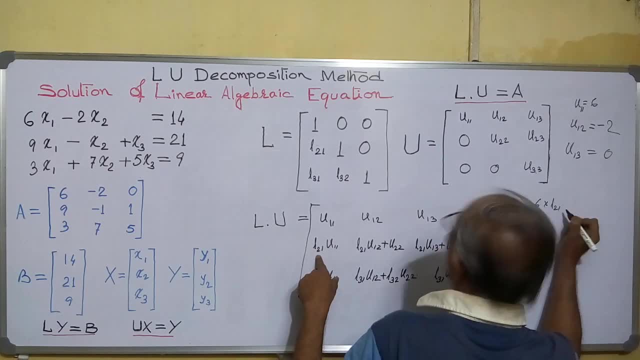 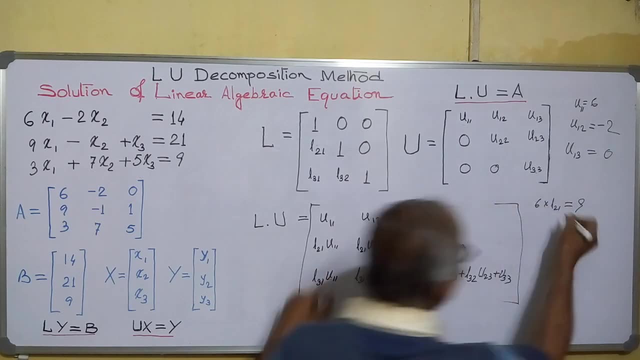 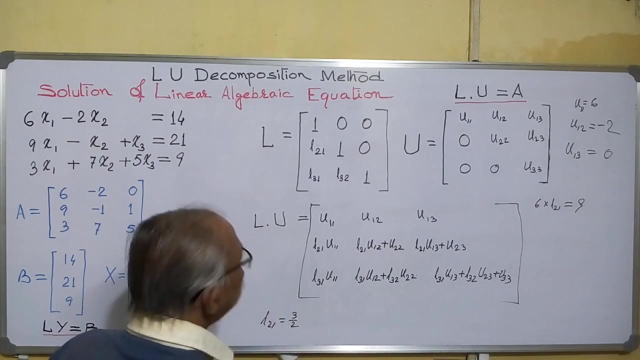 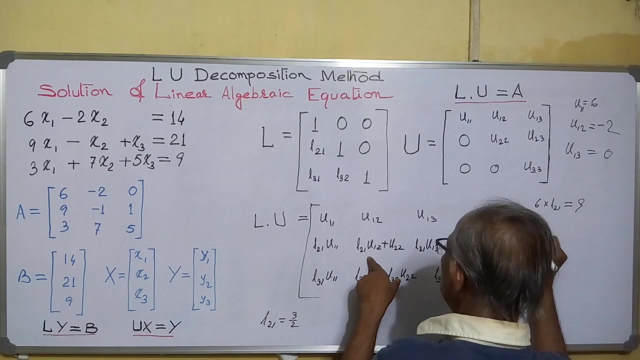 That is 6 into L21. We are getting 9. So that means L21 is 9 by 6. L21 equals to 3 by 2. Then L21, that is 3 by 2, into U12 minus 2.. 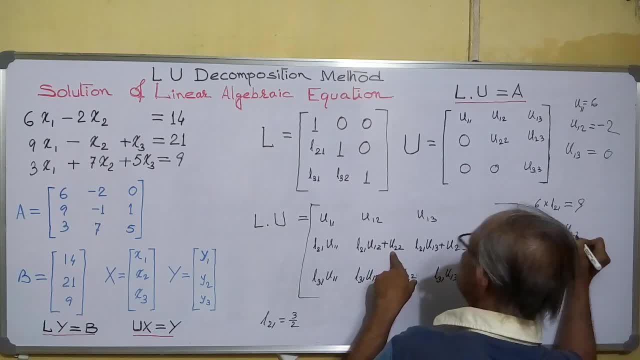 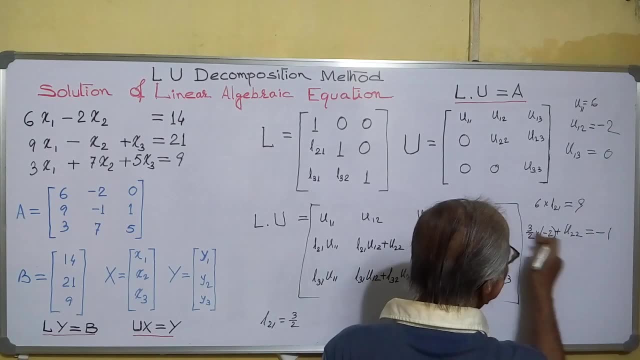 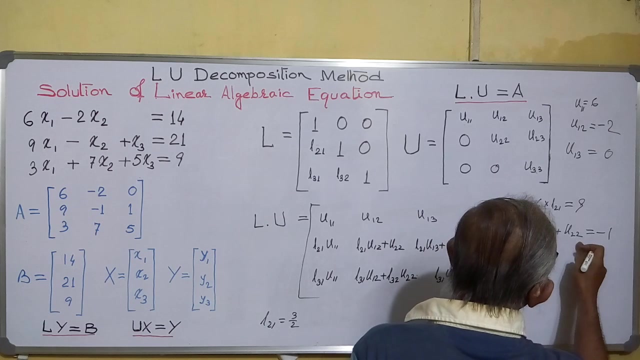 Plus U22.. This is equals to minus 1.. This is minus 3.. It will go that side, So it will become plus 3 minus 1.. U22 equals to 3, minus 1 equals to 2.. U22 equals to 2.. 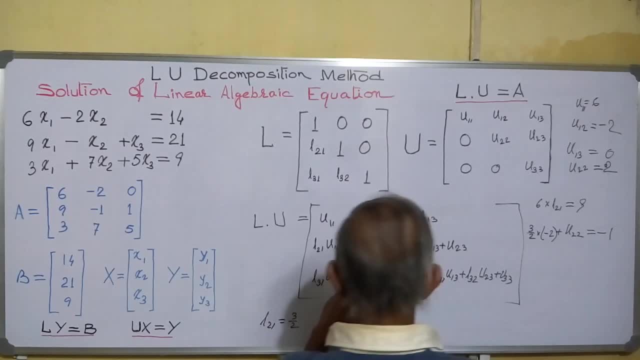 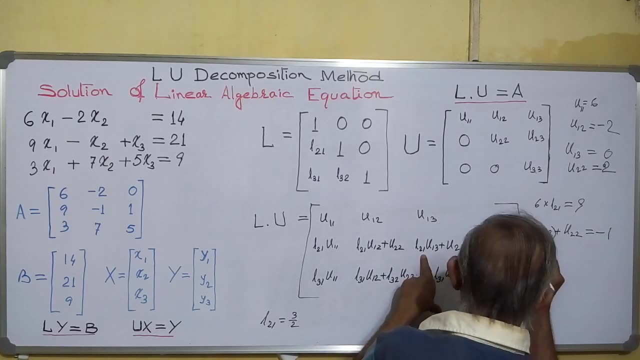 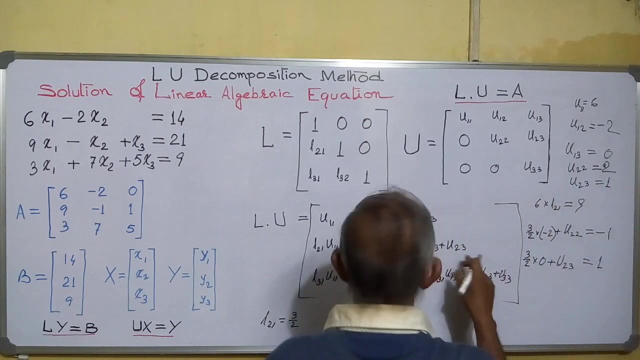 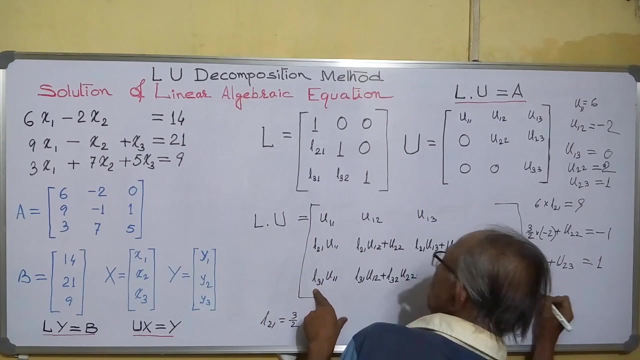 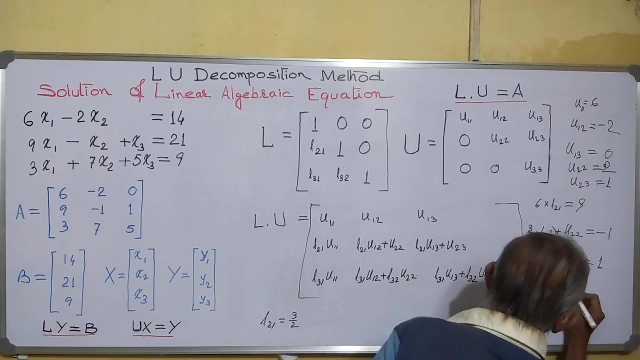 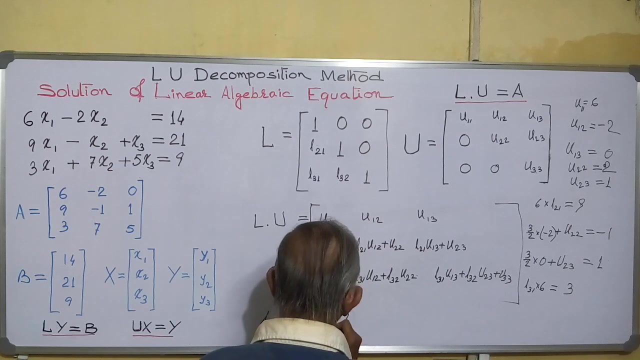 Then L22.. L21 is our 3 by 2 into u1 by 3.. u13 is 0 plus u23.. This is equals to 1.. That means u23 equals to 1.. Now L31.. L31 into u116 equals to 3.. That means L31 equals to 3 by 6.. That is L31. 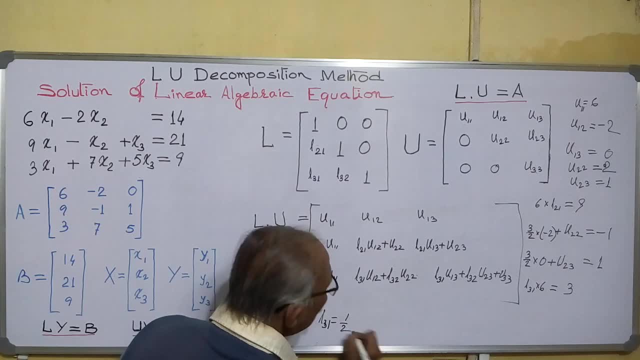 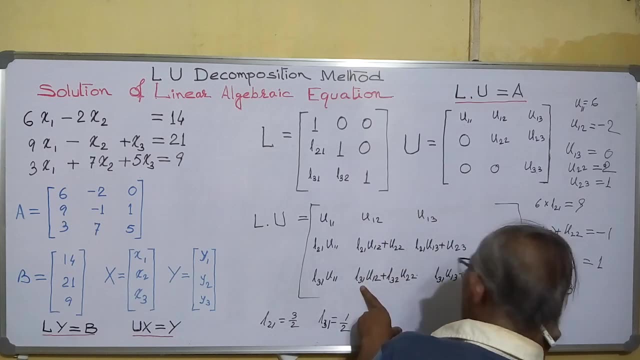 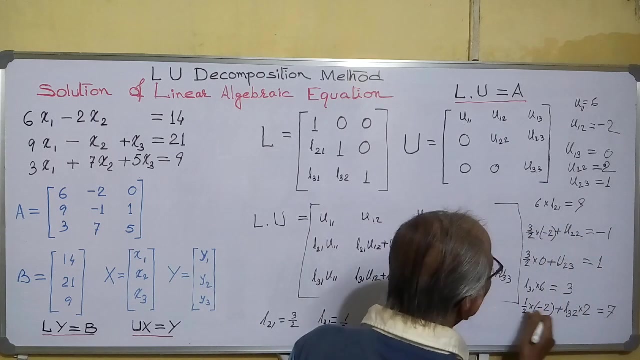 equals to 3 by 6.. L31 equals to half. Now L31, that is half into u12, is minus 2 plus L32.. Not known L32 into u22 is 2. equals to this element is 7.. So half into minus 2 equals to 3 by 6.. That 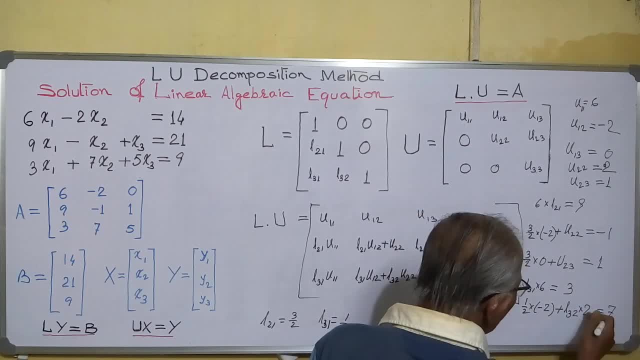 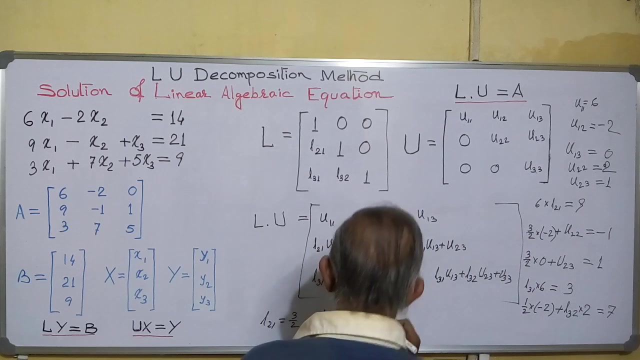 means L32 minus 1.. It will go that side. 8 by 2 will be 14.. So L32 is 7.. Half minus 2 minus 1.. Minus that, one will go That side, it will be 8.. 8 by 2 is 4.. L32 equals to 4.. 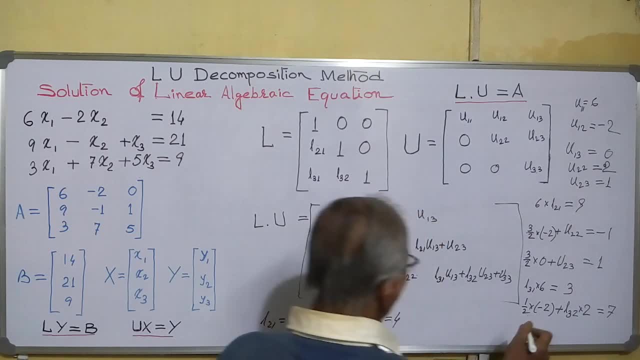 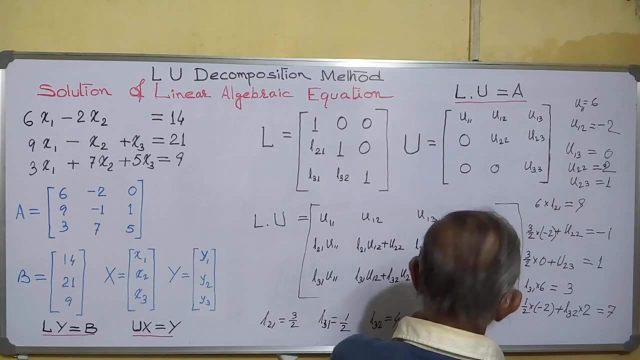 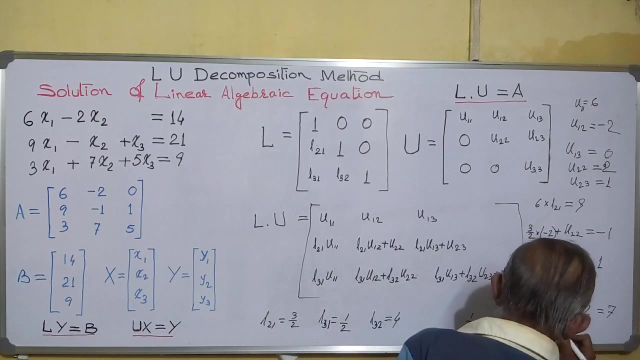 Then L31.. L31 is half into u13, is 0 plus L32 is 4 into u23 is 1 plus u33. This is equals to 5. So from 0, 5 minus 4 is 1.. So u33 is 1.. 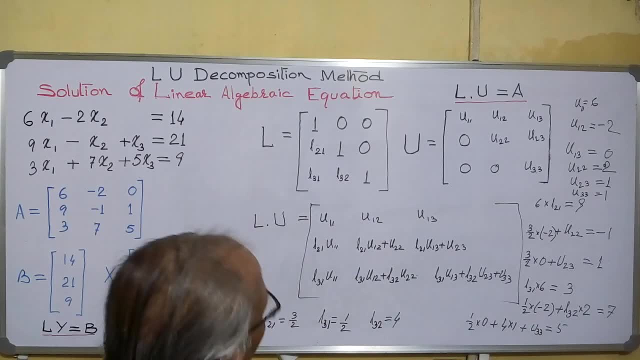 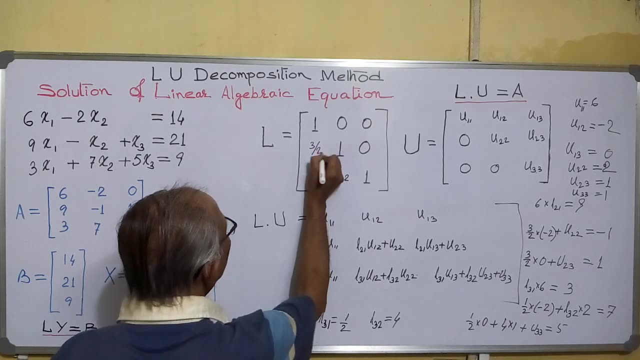 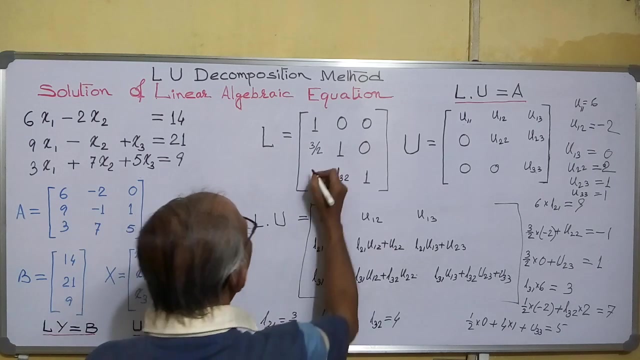 So now we will put these values here. What we are getting: L21 is 3 by 2.. This we are getting 3 by 2.. L31 is half. This is half. L32 is 4. And u11 is half. So this is half. 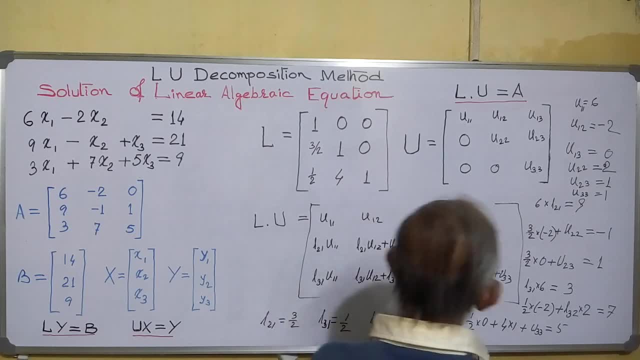 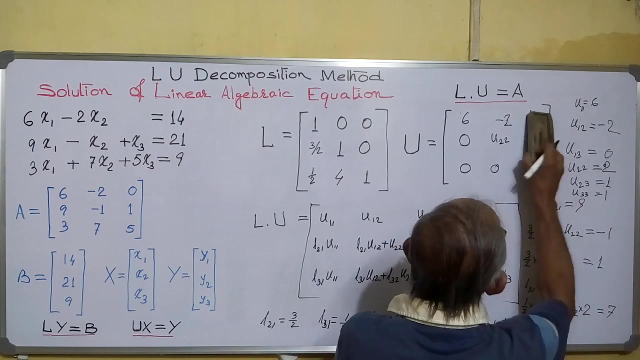 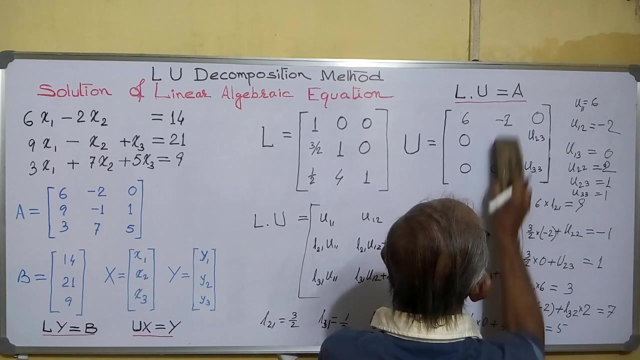 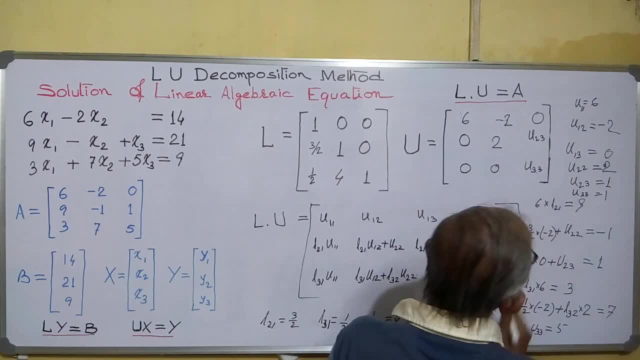 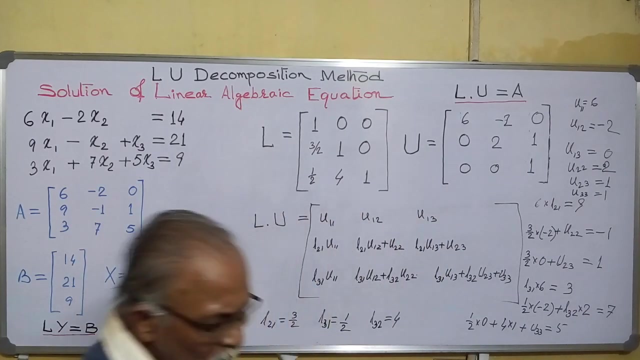 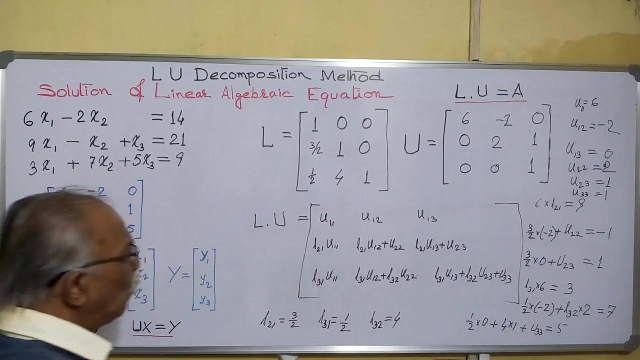 U23 is 1.. U33 is also 1.. It is 0.. This is 0.. That is same. So now, in this way, we are getting L and U with the assumption- our assumption- L into U equals to A. A was known. We have searched L and U. In this way, we are getting L and U. 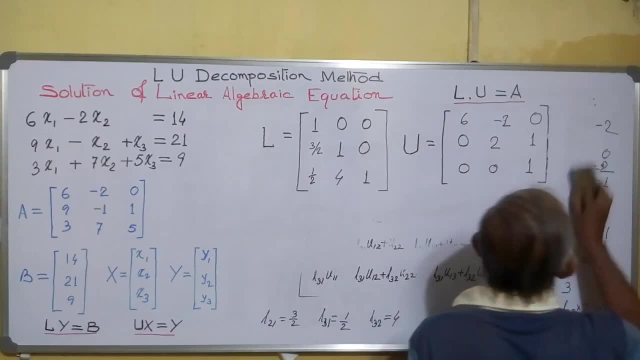 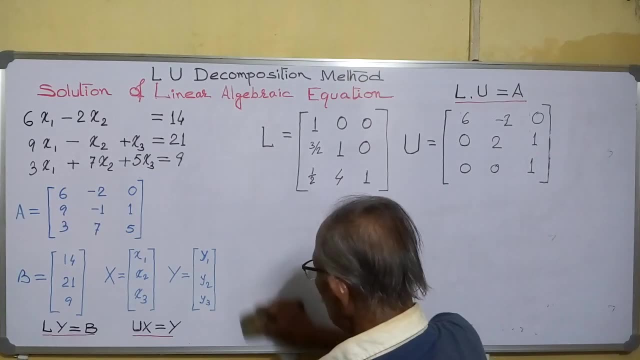 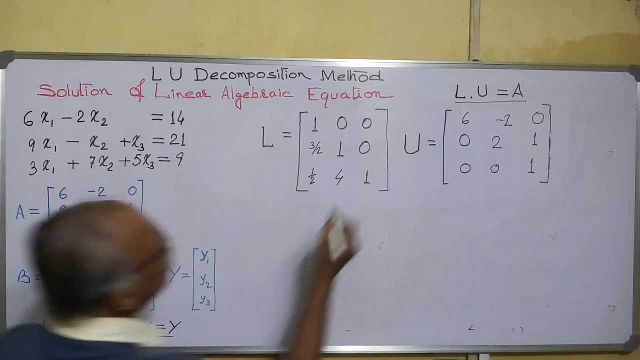 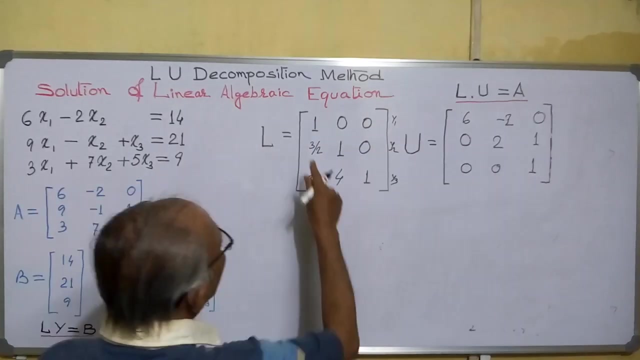 Now we have to proceed further with this After knowing L and U. With this, L Y equals to B, Y is about Y1, Y2, Y3.. I am showing here Y1, Y2, Y3. We have to try it properly. 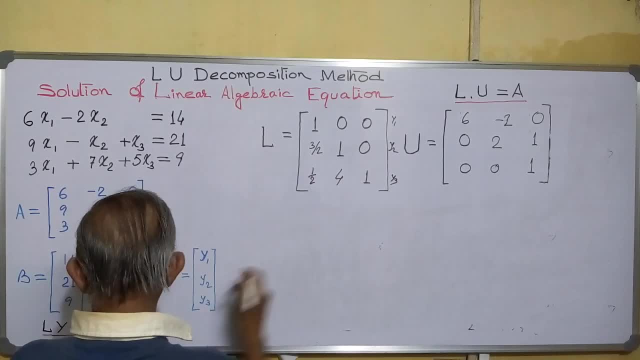 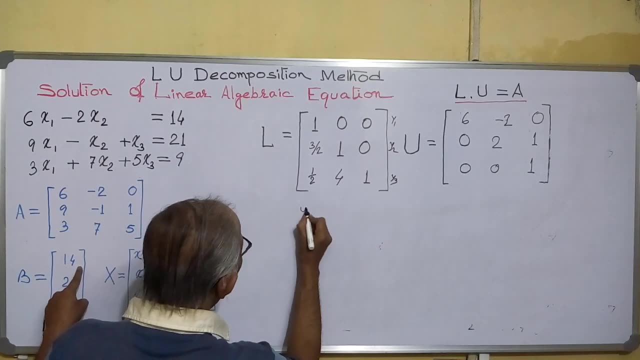 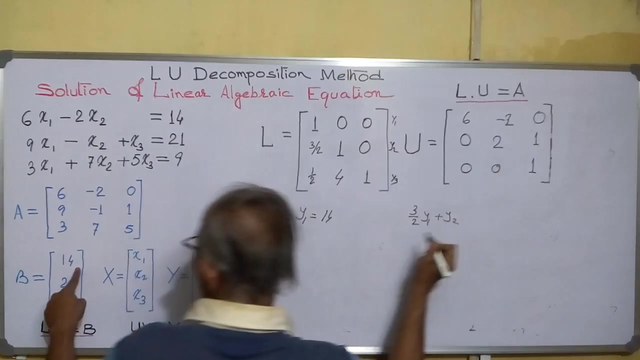 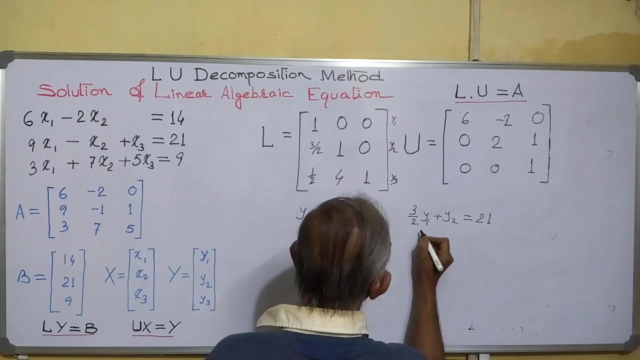 So L Y equals to B. This is our B. So 1 into Y1 equals to 14.. Then 3 by 2, Y1 plus Y2 equals to 21.. Now 3 by 2, Y1 in our 14.. 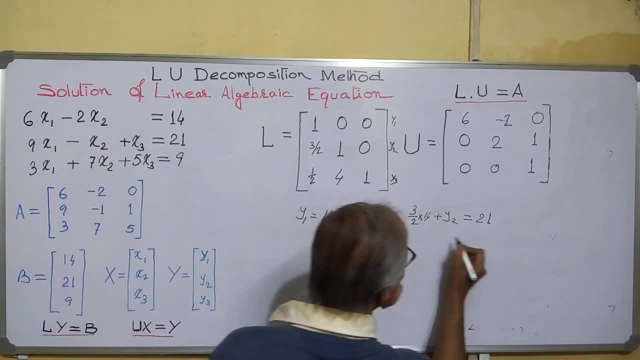 So 3 by 2, Y1 in our 14.. 3 by 2, Y1 in our 14.. 3 by 2, Y1 in our 14.. 7 by 2, 21, 21. So Y2 is becoming 0.. 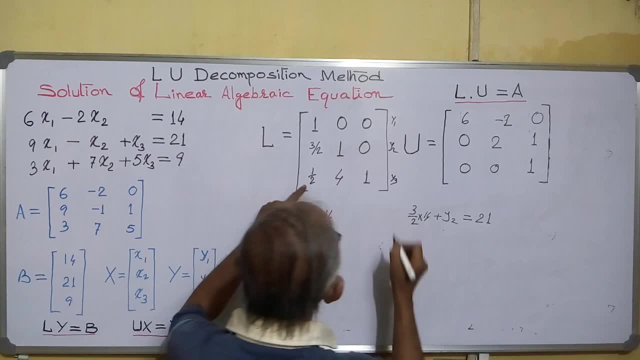 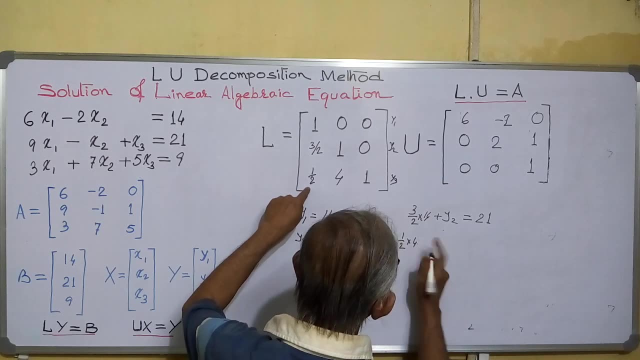 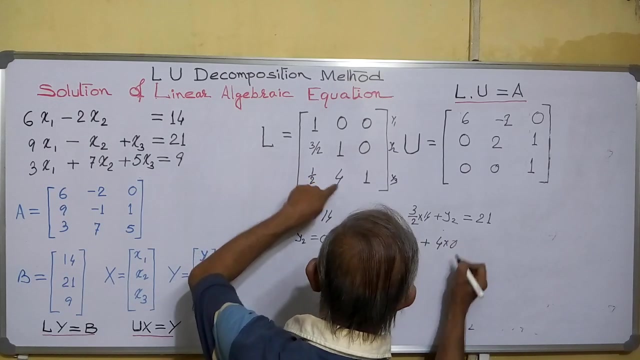 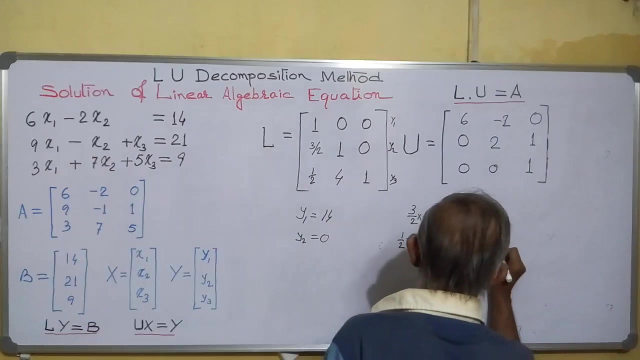 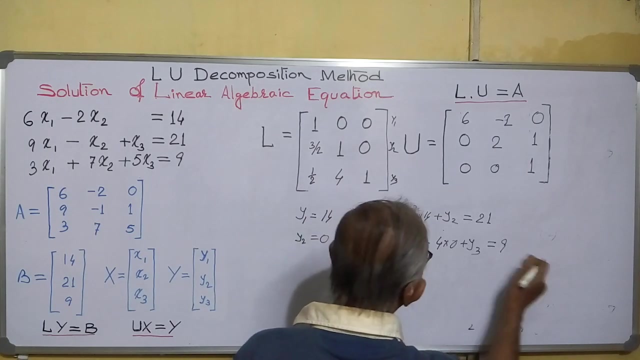 Now half Y1 is 14.. Half into 14 plus 4Y2.. 4 into 0 plus Y3. This one equals to 9.. So 7 is going that side. So 9 minus 7 is 2.. 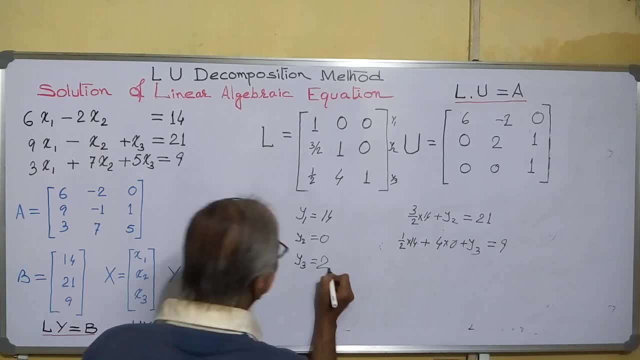 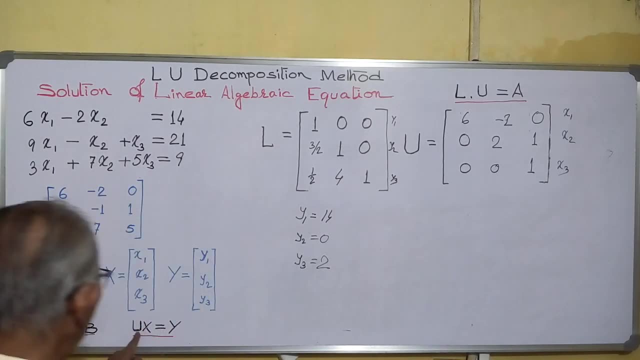 So we are getting Y3 equals to 2.. So in this way we got the matrix Y. Now we have to proceed: U into X equals to Y, U into this one equals to Y, Then Y, Then Y, Then Y. 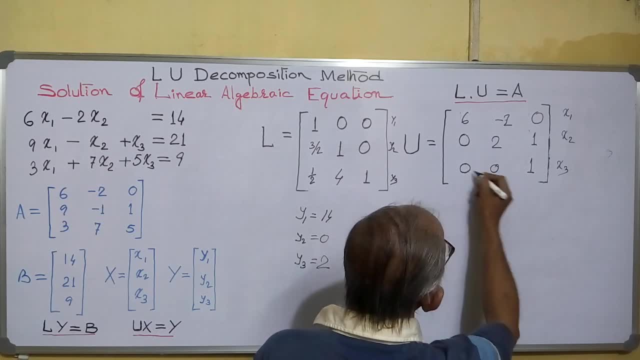 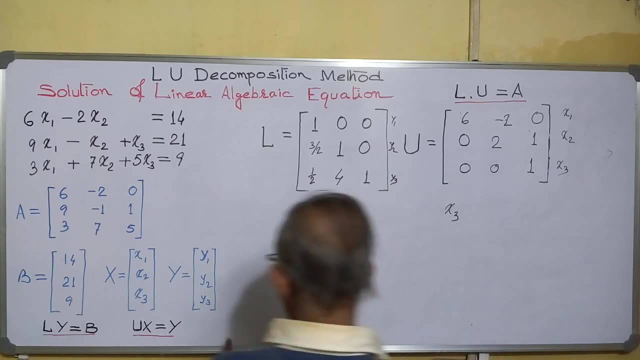 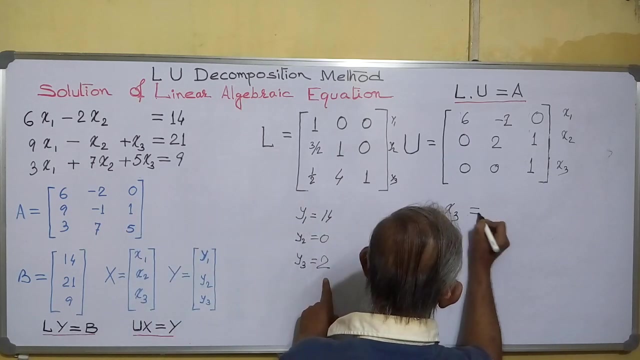 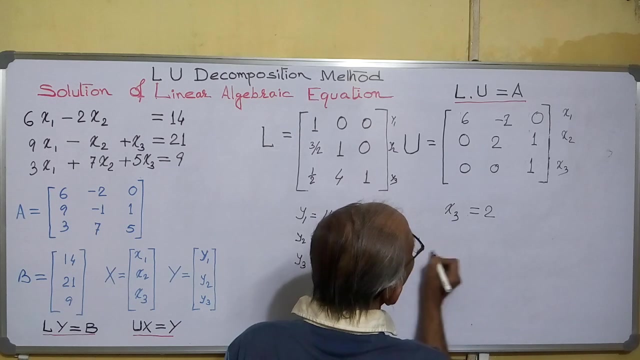 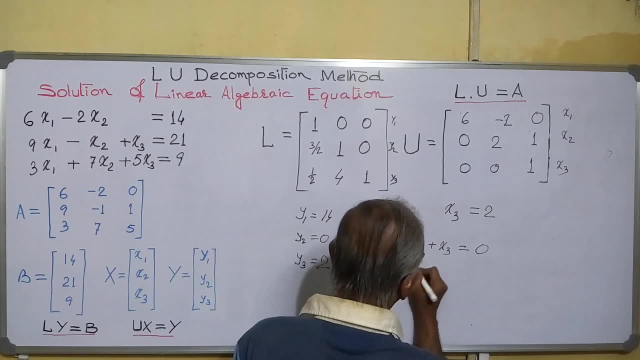 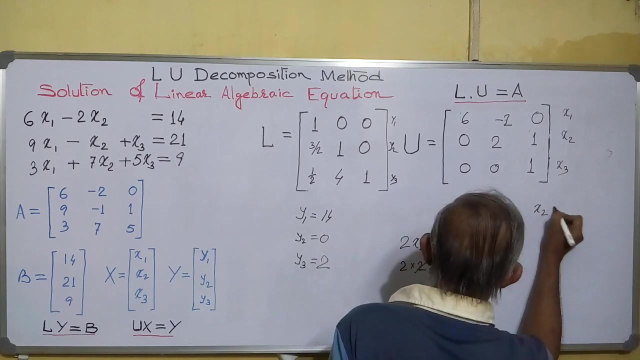 X3 is 2.. So 2 into 2.. 2 into X2 is 2 into X2. plus 2 equals to 0. So X2 equals to minus 1.. 2 will go that side. X2 will become minus 1.. 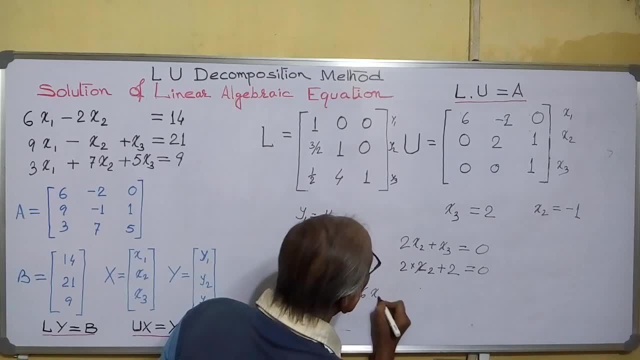 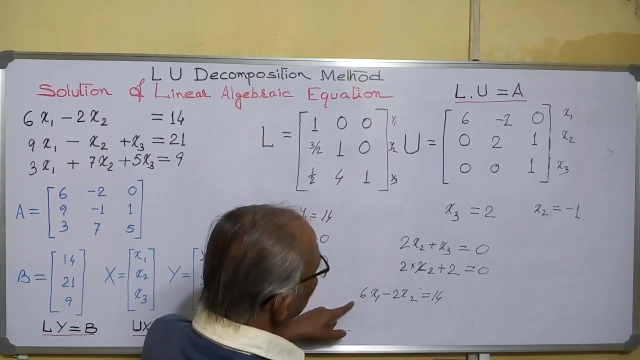 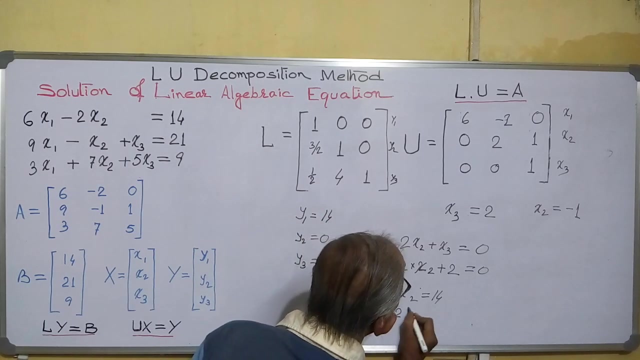 Next is this one: 6X1 minus 2X2 plus 0, is there? This one equals to 14.. Why That is 14.. Now 6X1.. 6X1 minus 2 into X2 is minus 1.. 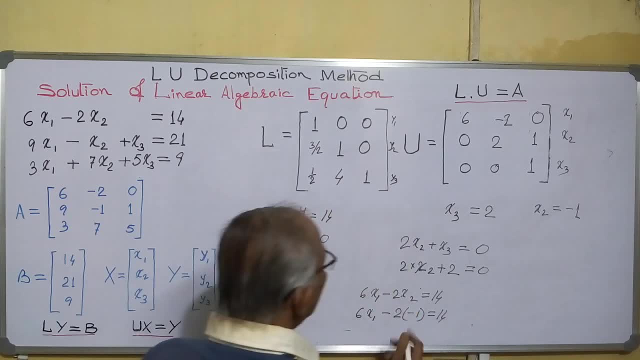 6X1 equals to 14.. That minus 2 into minus 1 plus 2 equal to will go that side, 14 minus 2 will 12.. 6X1 equals to 12. So X1 equals to 2.. 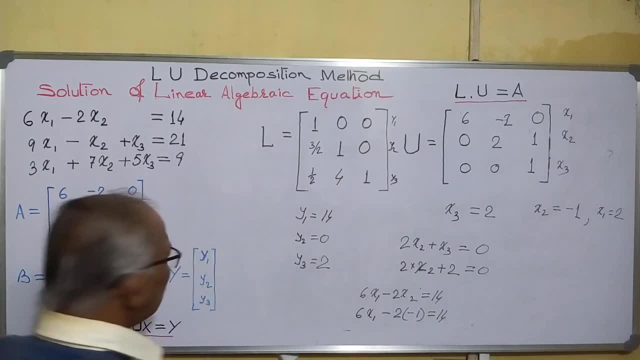 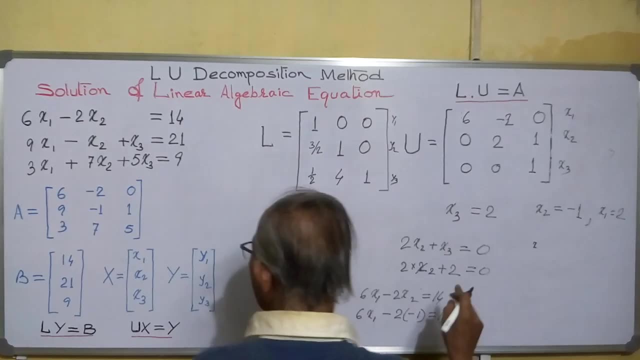 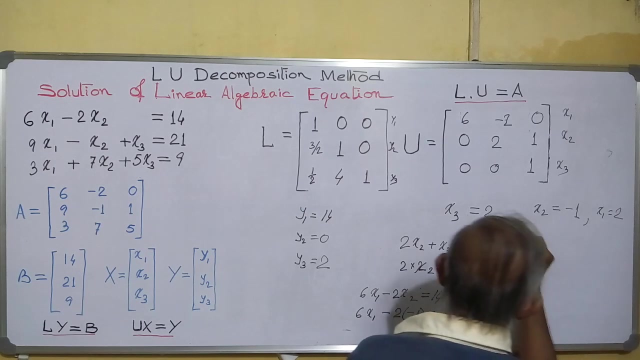 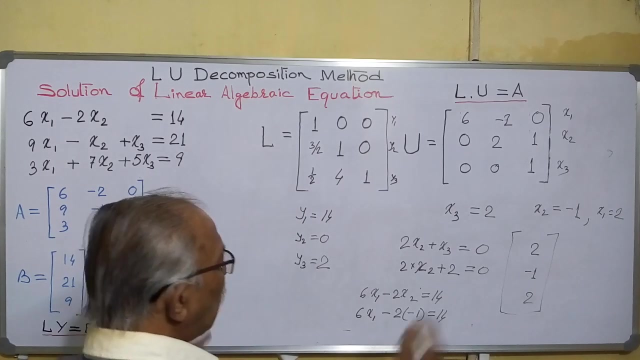 In this way we can get the matrix X That is. our required solution is 1X1.. This is the matrix that is open. So X2 equals to 2X3 equals to 2.. X1 equals to 2.. X2 equals to minus 1..